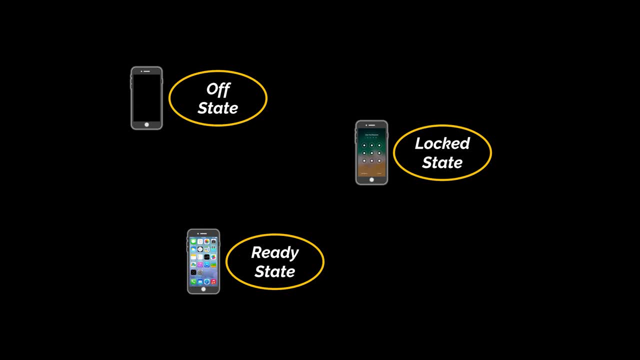 different states: the off state, locked state and ready to use state. When we first grab our phone, it's turned off. To turn it on, we can use both the power button or the home button, But either way our phone will still be locked. we can't access our applications yet. To do this, what we need, 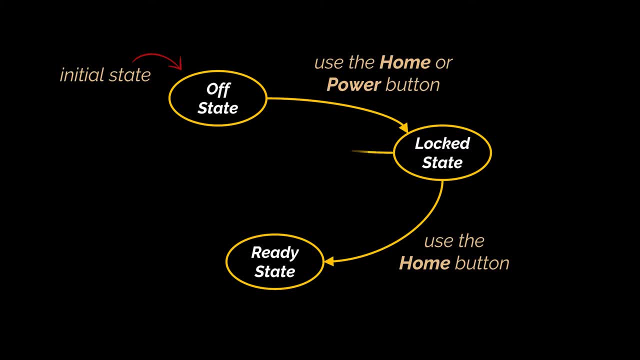 is to click a second time on the home button. We can't use the power button this time to turn it off. And finally, while using our phone, we can at any time use the home button to access the home page or use the power button to turn it off again. 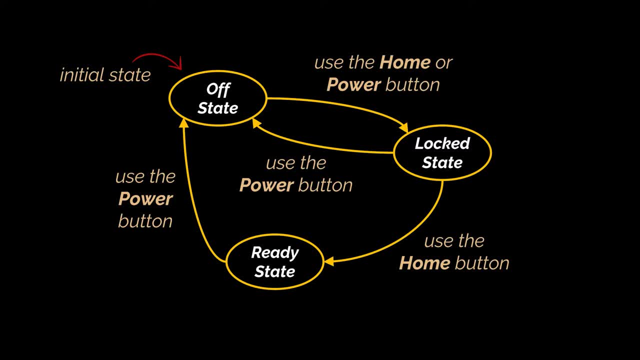 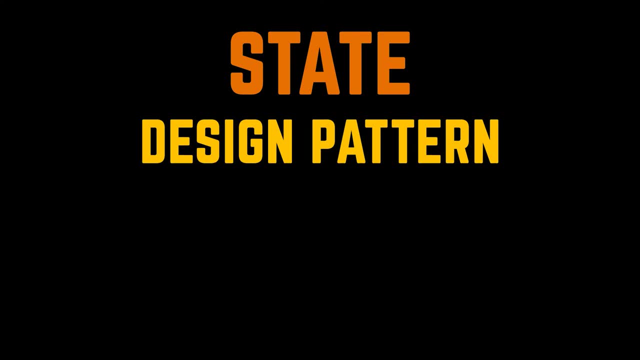 What we just drew is this state machine of our previous example, Easy right. This concept is closely related to, and usually associated with, the state design pattern. The state pattern is a behavioral design pattern that lets an object alter its behavior when its internal state changes. 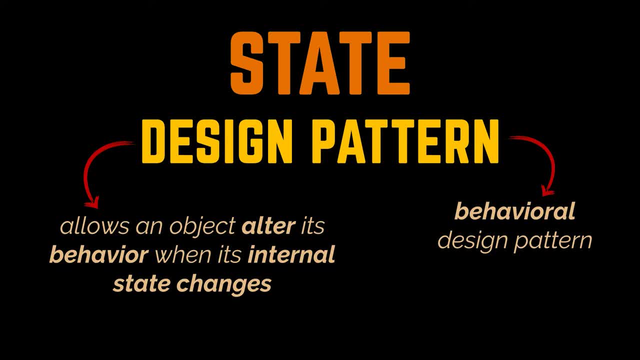 It may seem as if the object changed its class. To dive deeper in this definition, let's try and implement together the phone example we had using the state design pattern. The first thing we need is a context. What is the object that changes states? 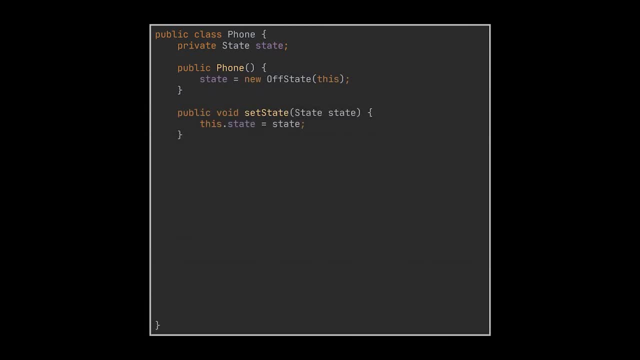 In this case it is the phone, so we can have a phone class. This class will house the state of the phone, obviously among several additional methods, which are the functionalities this phone can perform. For the sake of the example, we will just be returning a string or two. 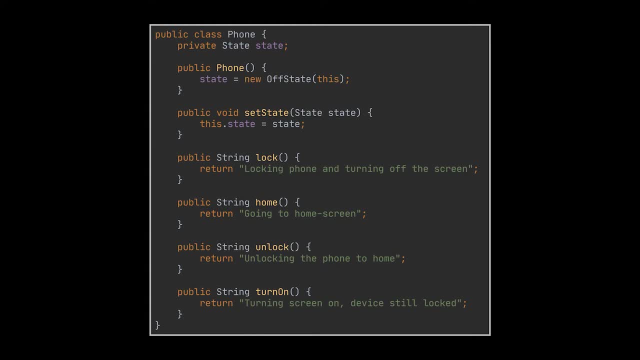 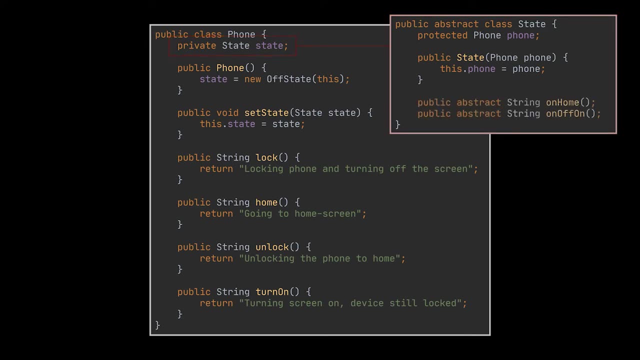 Now the state class we have here will be an abstract class which stores an instance of the phone it is acting on, and two methods, each representing one of the buttons. we have One representing what will happen when we click on the home button, and the second what 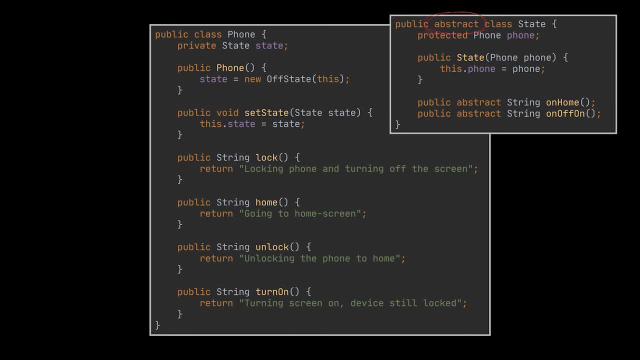 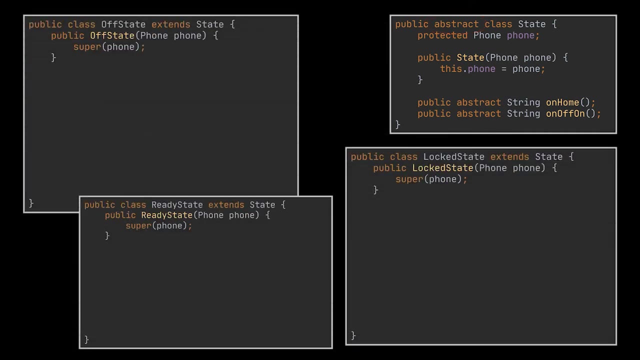 will happen when we click on the power one. We mentioned that this class should be abstract right, And that's because the actual states of our phone will each be represented by a different class that extends this one. In our case, we will have three classes, one for each state, so the off state, the locked, 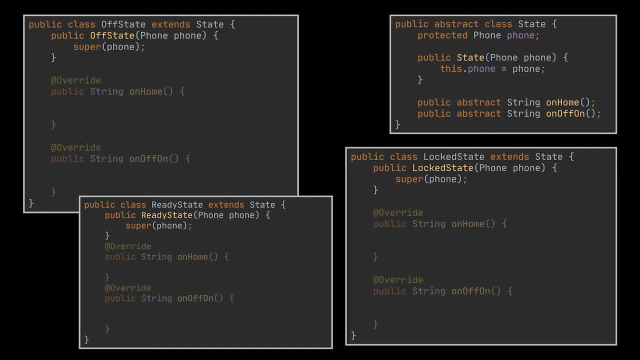 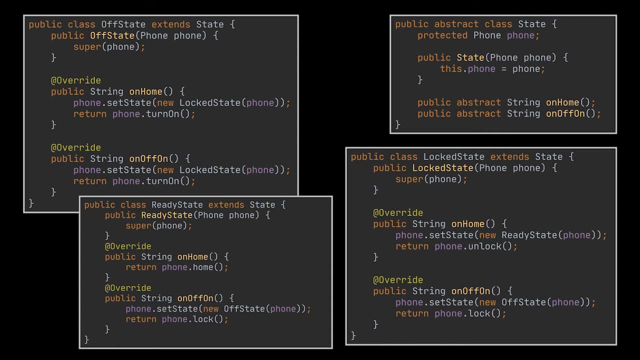 state and the ready state classes. Now each state class will have to override these two abstract methods, and the actual implementation can consist of jumping to another state, like we saw on the state machine diagram, and or invoking one or several of the functionalities we implemented in the 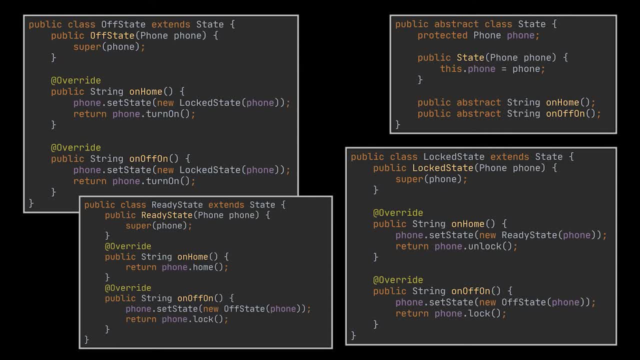 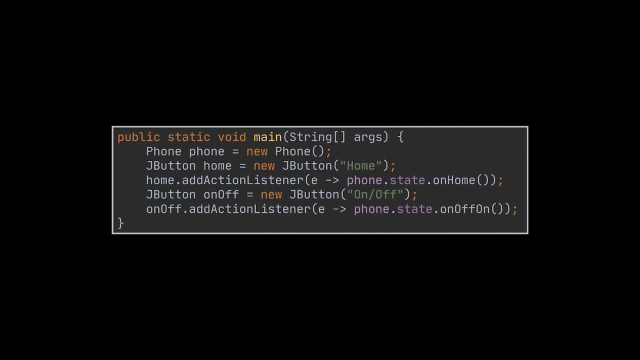 phone class. And that's it: our different phone states implemented using the state pattern. On top of that, To simulate this, you can imagine you have J buttons with the listener tied to its respective abstract method. Then, based on the phone state, when a user clicks on any of the two buttons, the corresponding 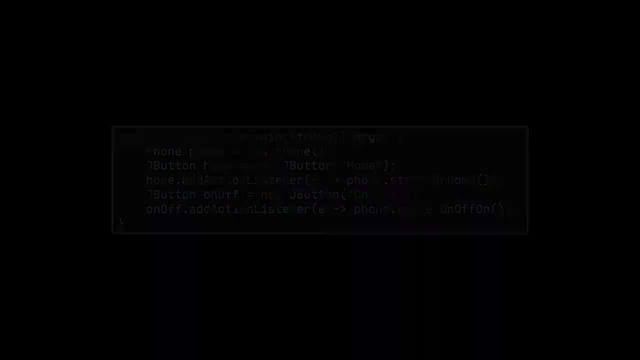 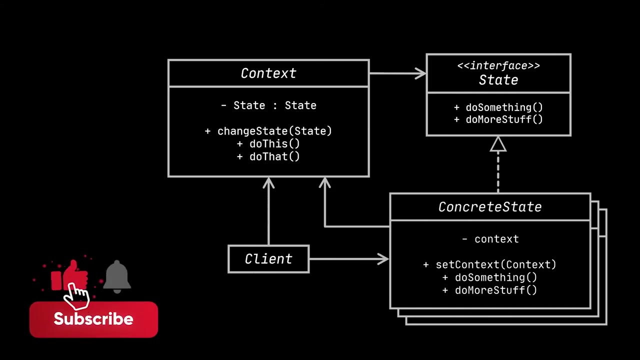 behavior will be called. Now, I know most people confuse this pattern with the strategy one, and I'll compare them in a bit, but before doing so, let's take a look at the structure or class diagram of the state pattern, while relating it to the phone example we just implemented. 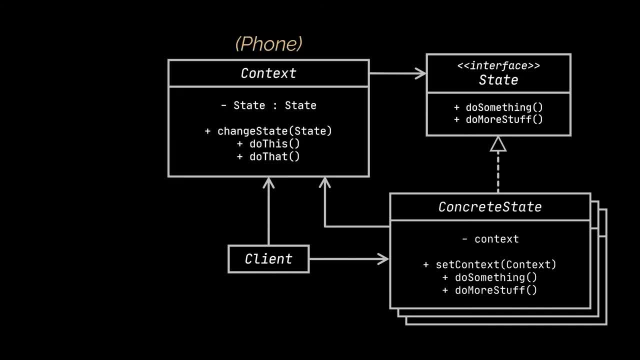 The first thing you may notice Is the context class, which was the phone class in our previous example. The context stores a reference to its current concrete state, initialized as the initial state the context is supposed to start with. The context communicates with the state objects only via the state interface or abstract class. 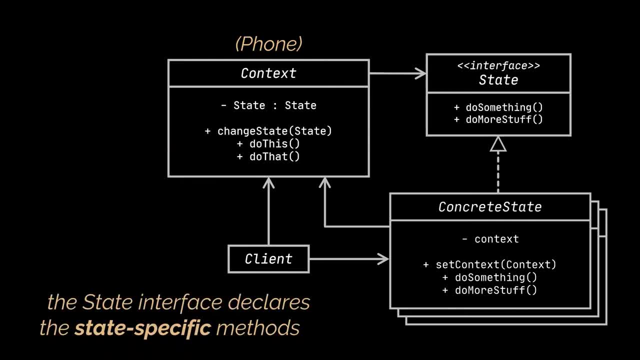 On the other hand, the state interface or, in our previous example, the abstract class, declares the state-specific methods. These methods should make sense For all concrete states, because you don't want some of your states to have useless methods that will never be called. 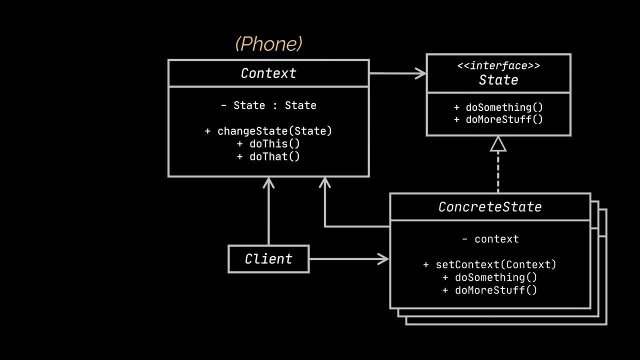 The next classes in our diagram are the concrete states, which were represented by the off state, the locked state and the ready state classes. These classes provide their own implementation for the state-specific methods. To avoid duplication of similar code across multiple states, you may encapsulate some. 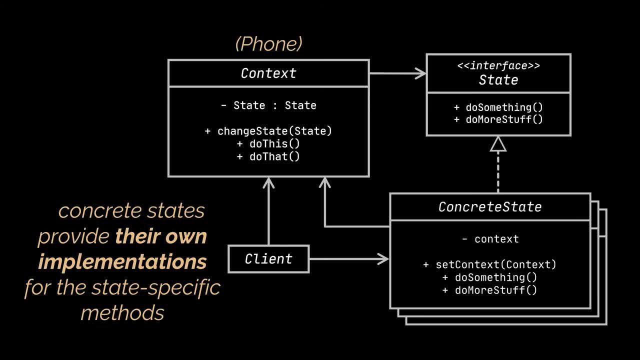 common behavior in an abstract class. Both the context and concrete states can modify the state-specific methods. Both the context and concrete states can modify the state-specific methods. Both the context and concrete states can modify the state-specific methods Kind of like this: 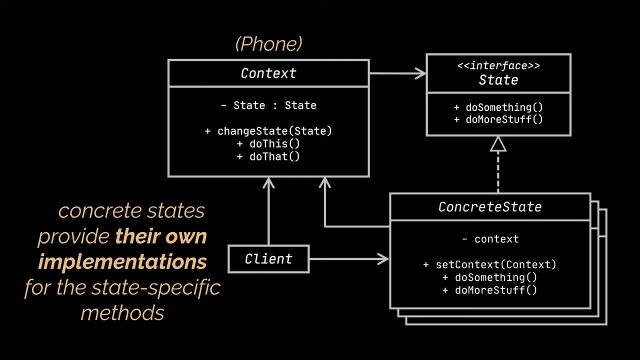 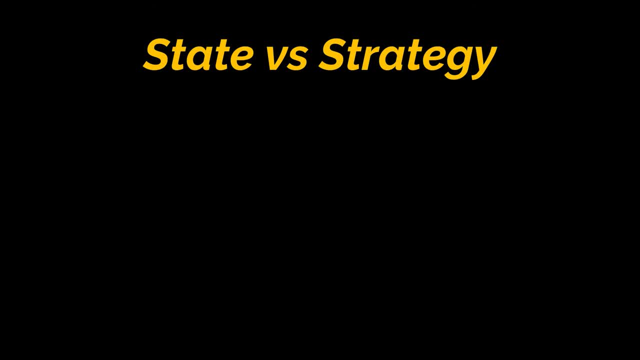 They must identify the state of the context or perform the actual state transition. Now, before ending the video, I want to tackle the difference between the state and the strategy patterns. You see, the state can be considered as an extension of strategy, as both patterns are. 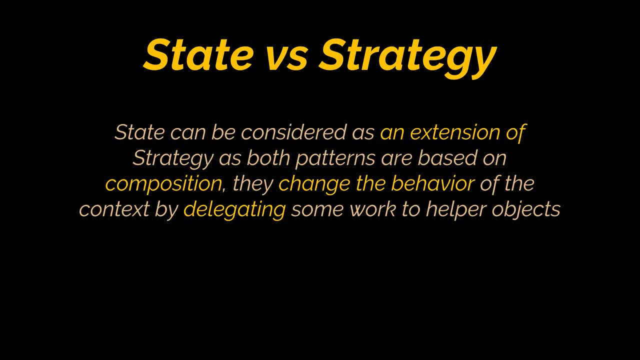 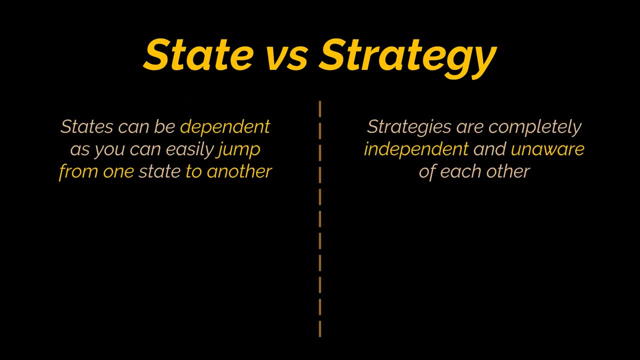 based on composition. They change the behavior of the context by delegating some work to helper objects. However, strategies are completely independent and unaware of each other. Both states can be dependent. You can test how the context или the strategy 2006 stops the state or the complex.